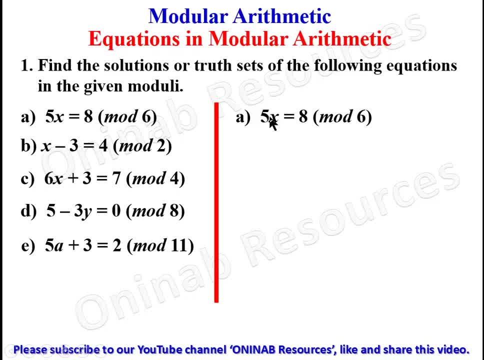 A5x is equal to 8 mod 6.. Here what we do is to look for multiples of 6, because we are working with modulo 6.. So we look for multiple of 6, such that when added to 8, the sum will be divisible by 5. So the multiple of 6 is 12.. So we have it as 8 plus 12 mod 6.. 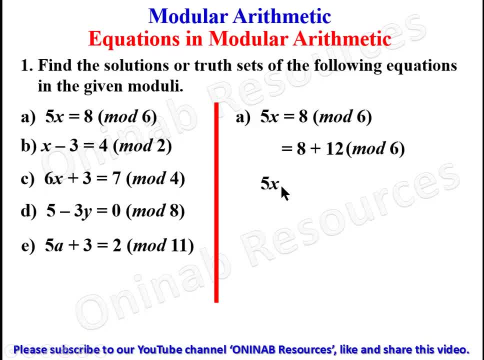 8 plus 12 is 20.. So 5x is equal to 20 mod 6.. 20 divided by 5 gives 4.. So x, x is equal to 4 mod 6.. We stop here and go to problem B. 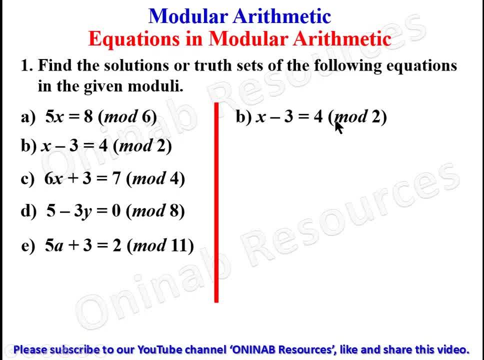 Problem B: We have x minus 3 is equal to 4 mod 2. So we subnormally take this negative 3 to the right hand side. So we have x is equal to 7 mod 2. Since 4 plus 3 gives 7.. 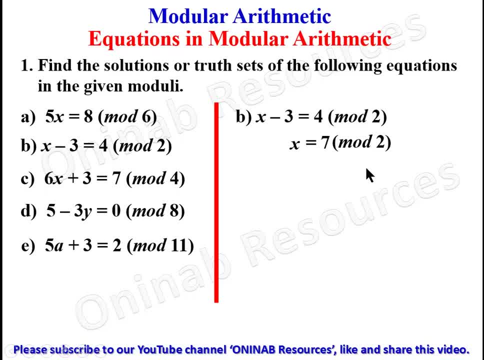 So x is 7 mod 2.. And here we can just find the equivalent modulo of 7 in mod 2. That is going to give us 7 divided by 2 gives 3 remainder 1.. So our x will be equal to 1 mod 2.. 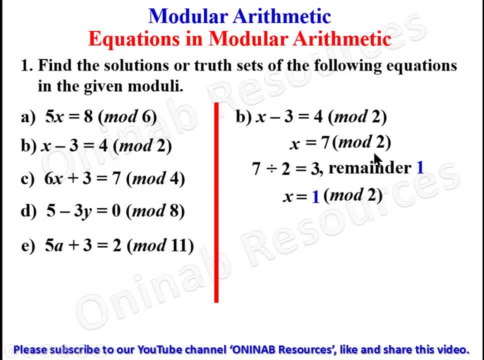 Our x is equal to 1 mod 2. You can also just subtract multiple of 2 from 7 to get 1.. That is 6.. It would have just been 7 minus 6. It gives 1 mod 2.. 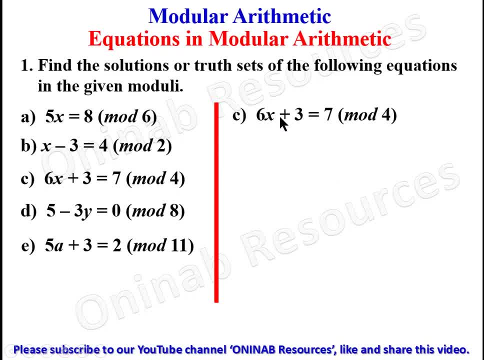 So we go to problem C: 6x plus 3 gives 7 in mod 4.. So we take this 3 to the right hand side, It becomes negative. So we have 6x equal to 4 mod 4.. 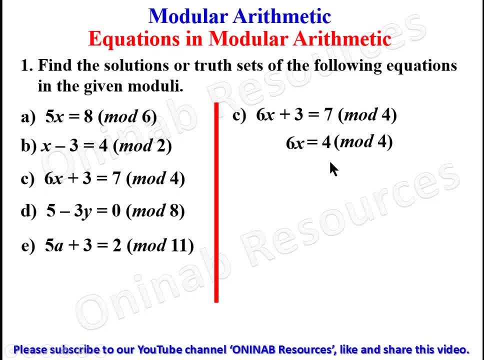 And we look for equivalent modulo of 4. Such that it is divisible by 6 by adding multiple of 4. And 4 plus 8. 8 is a multiple of 4. Plus 8 will give us 12.. So 4 is 12 mod 4.. 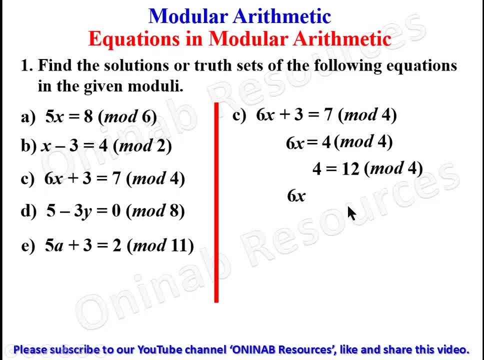 So therefore we now have: 6 is equal to 12 mod 4. So 12 divided by 6 gives 2.. So x is equal to 2 mod 4.. So we go to problem 1D. 5 minus 3y is equal to 0 mod 8.. 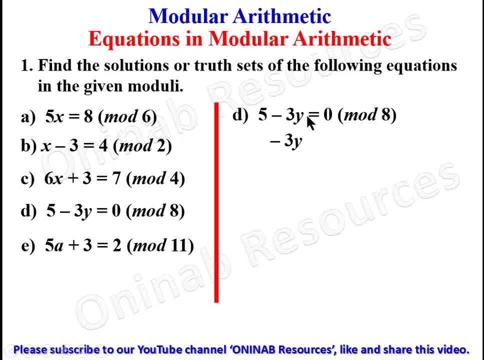 So we have negative 3y is equal to negative 5 mod 8.. After taking this 5 to the right hand side, So we still have it as 3y is equal to 5 mod 8.. After dividing both sides by negative 1.. 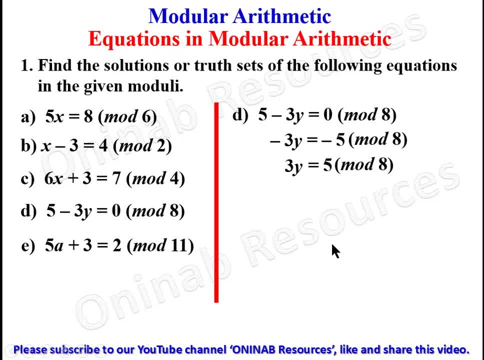 So here again, Um 5 is equal to adding multiple of 8 to 5. We have 5 to be equal to 21 mod 8.. 21 mod 8.. The multiple of 8 that we have added is 16.. 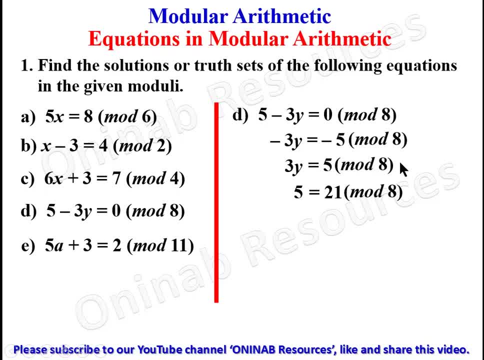 So therefore 3y is equal to 5 mod 8. Plus 3y is equal to 21 mod 8. And 21 is divisible by 3. So y is equal to 7 mod 8. Dividing 21 by 3 gives 7.. 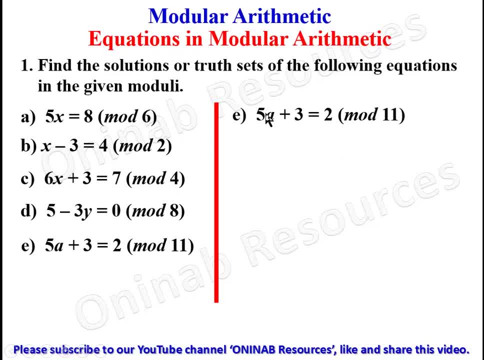 So we go to problem 1E. For problem 1E I have: 5a plus 3 is equal to 2 mod 11.. So what we do? we said 5a is equal to negative 1 mod 11.. 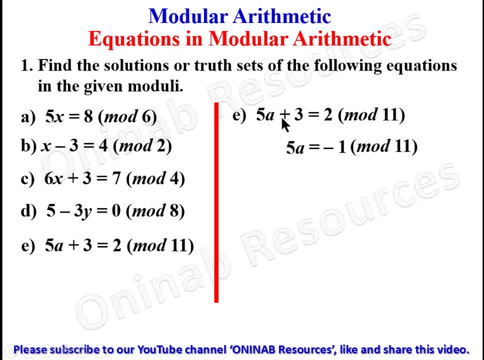 2 minus 3.. Since when you take this positive 3 to the right hand side It gives negative, So that point it becomes 2 minus 3, which gives negative 1 mod 11.. Now negative 1 is equal to negative. 1 plus 11 gives 10.. 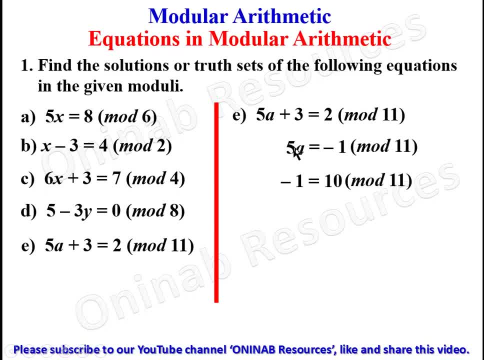 So that will give us 10 mod 11.. Since 10 is divisible by 5. So our equation becomes: 5a is equal to 10 mod 11. Which gives a equal to 2 mod 11. So that's the solution of problem 1E. 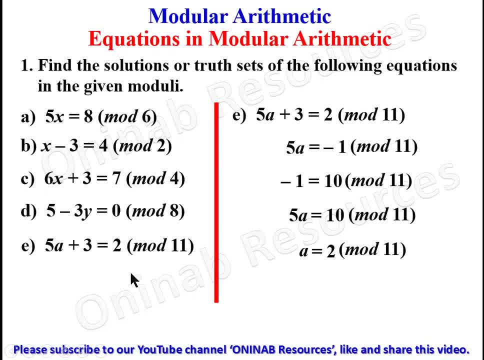 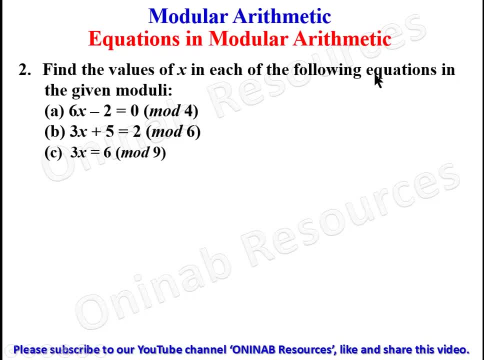 And that is all for problem 1.. We go to problem 2.. For problem 2.: Find the values of x In each of the following equations In the given moduli. Here we are not just finding one value of x. 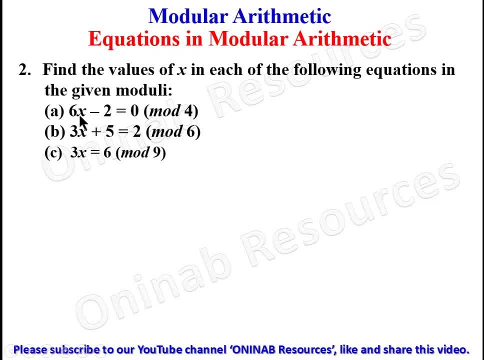 Find the values of x Meaning. there are many values of x that will satisfy each of these equations. So we start with a part of the problem. So we are taking this to the right hand side. We have: 6x is equal to 2 mod 4.. 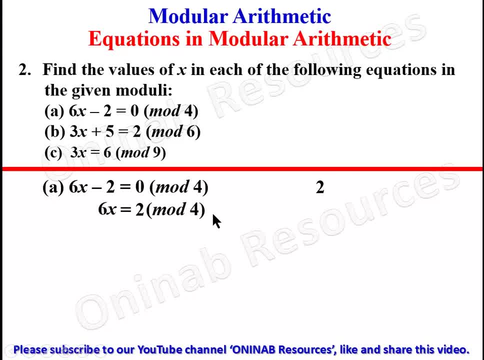 So we now bring this to and find its equivalent, modulo 4.. We want to see its equivalent modulo 4.. By continuing adding 4, we get the equivalent modulo, And we will now select which one will be divisible by 6. So we have 6 mod 4.. 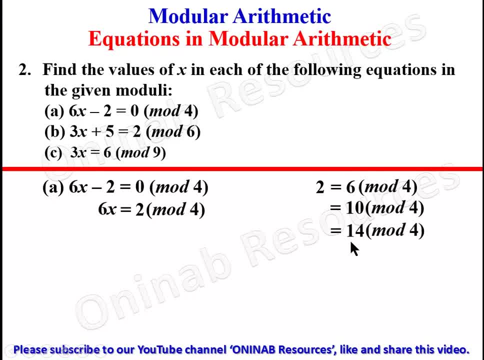 10 mod 4.. 14 mod 4.. 18 mod 4.. And this one is divisible by 6.. This is divisible by 6.. So our first set of solution will now be: 6x is equal to 6 mod 4.. 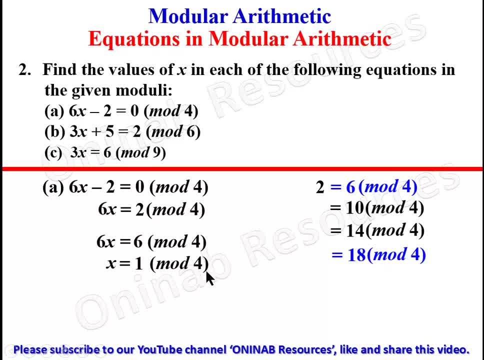 Where x is equal to 1 mod 4.. Again, 6x is equal to 18 mod 4.. And at that point x is equal to 3 mod 4.. 18 divided by 6 gives 3.. So these are the values of x which satisfy the equation. 6x minus 2 is equal to 0 in modulo 4.. 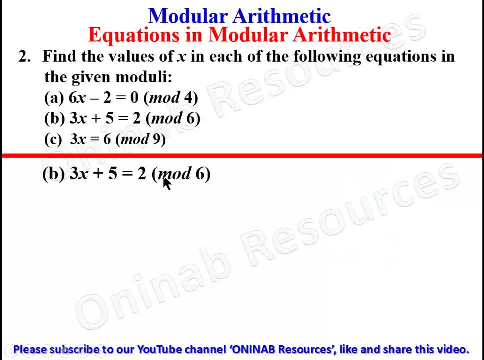 So we go to b For b I have: 3x plus 5 is equal to 2 mod 6.. So I Collect the like terms: 2 minus 5 gives negative 3 mod 6.. And again we get equivalent of 3 modulo 6.. 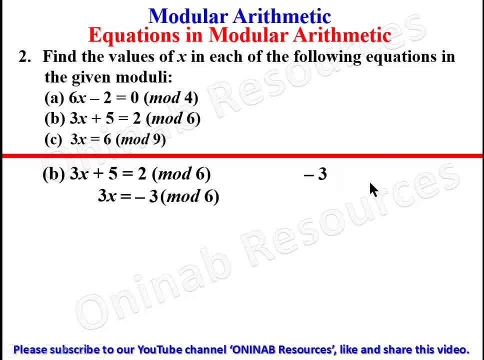 By continuing adding 6.. I have 3 mod. 6 adds 6.. Again, I have 9 mod 6. Add 6, I have 15 mod 6. If I add 6, I have 21 mod 6. And 21 divided by 3 gives 7.. 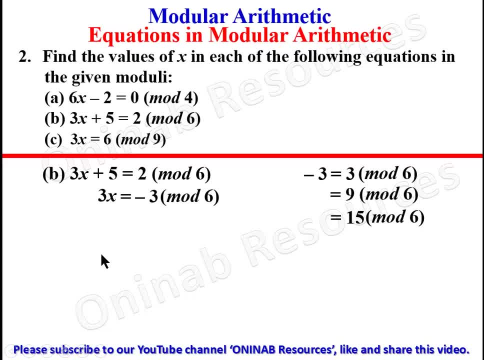 So we stop here. So our first set of solution will be: 3x is equal to 3 mod 6.. x is equal to 1 mod 6.. 3 divided by 3 gives 1.. Then the second set of our solution is: 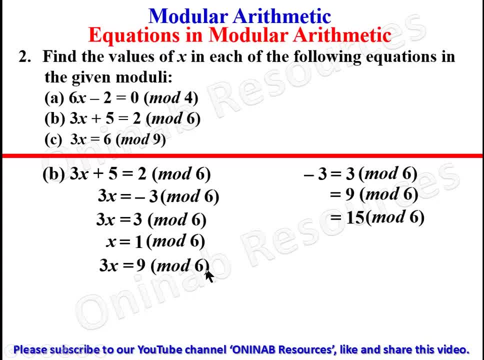 3x is equal to 9 mod 6.. Since 9 is divisible by 3.. That will give us: x is equal to 3 mod 6.. And finally, 3x is equal to 15 mod 6.. And x is equal to 5 mod 6.. 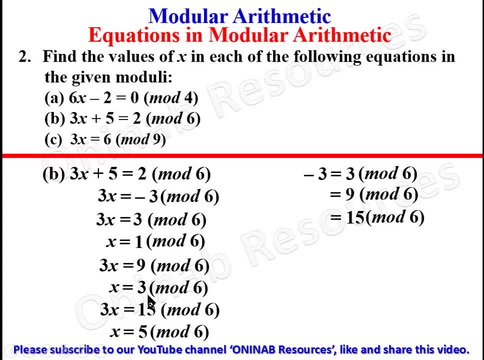 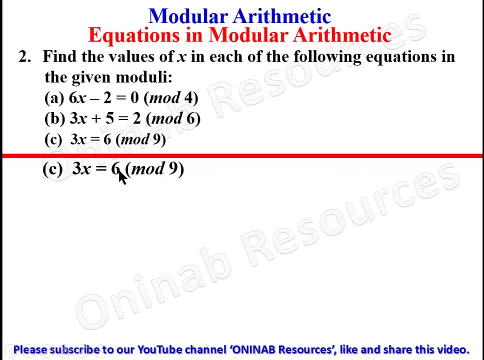 So the values of x are 1,, 3 and 5. Which satisfy the equation. 3x plus 5 is equal to 2 mod 6.. So we go to C part of the problem. 3x is equal to 6 mod 9..